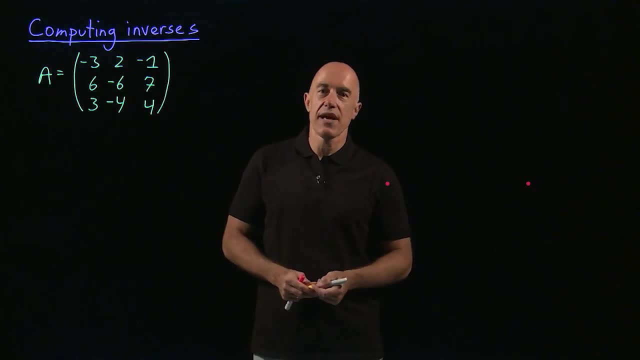 So we learned about the reduced row echelon form of a matrix. So in this video I can give you one practical application of that, which is to find the inverse of a matrix. So as the example I'm going to work. we have this matrix, A given here. Remember, not all matrices. 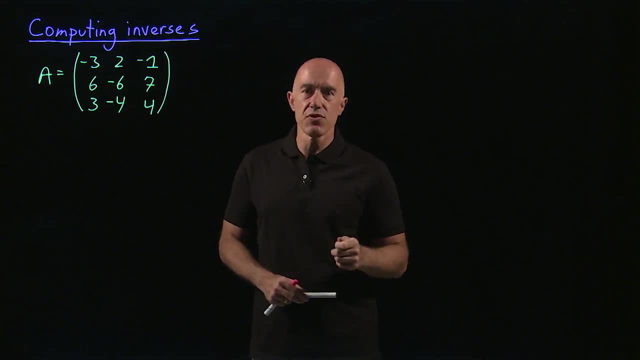 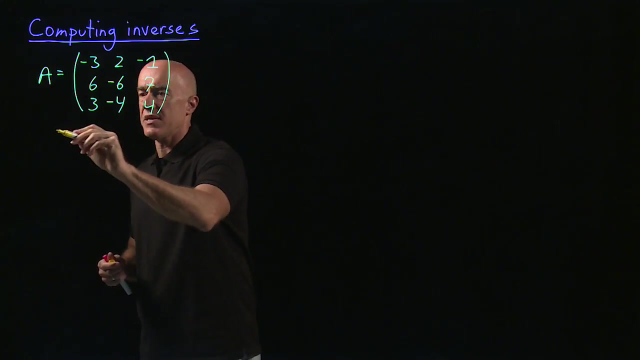 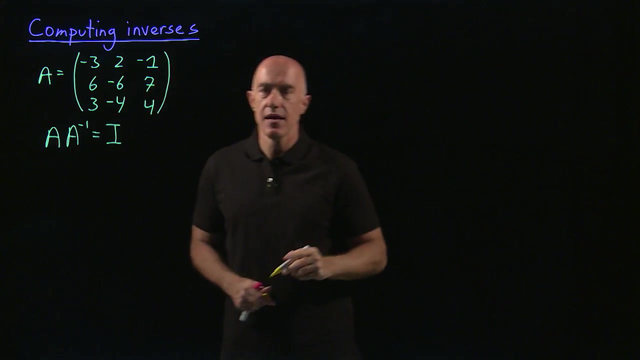 have inverses, but some of them do. They have to be square matrices. This one has an inverse. So the question here: how do we compute the inverse of this matrix? So what is the meaning of an inverse? So A times A inverse is supposed to be the n by n identity matrix. 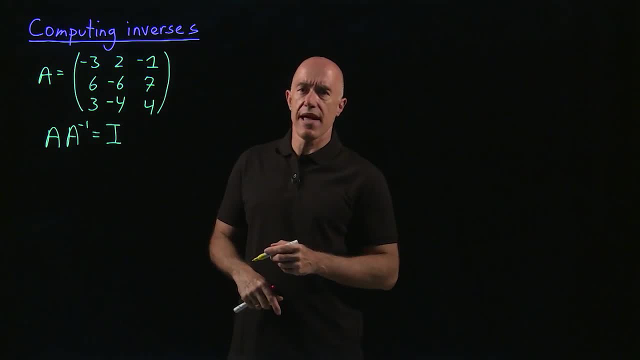 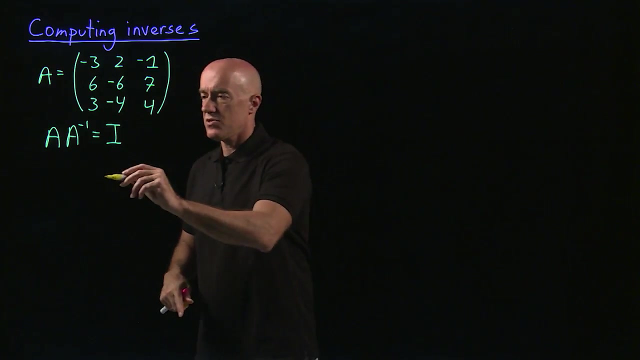 So here we have multiplication of two n by n matrices. But you can view this as the A matrix multiplying The first column of A inverse, giving you the first column of I, Then the A matrix multiplying the second column of A inverse, giving you the second column of I, et cetera for n columns. 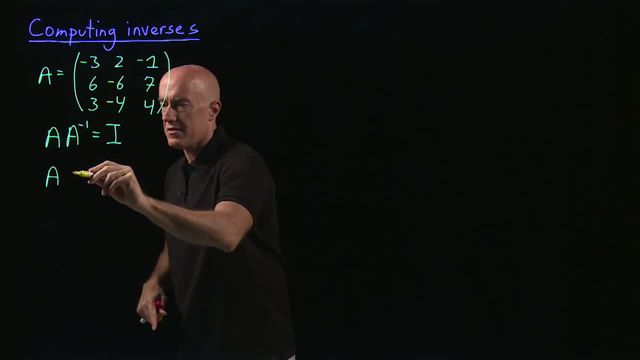 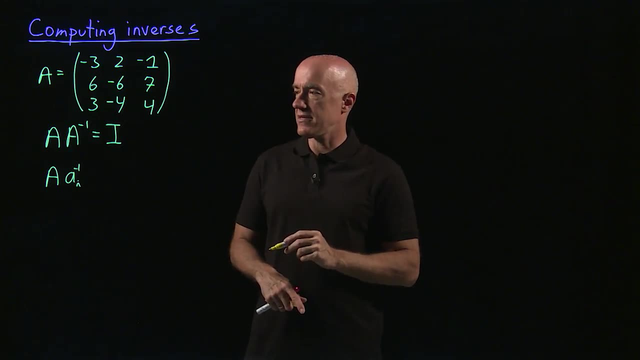 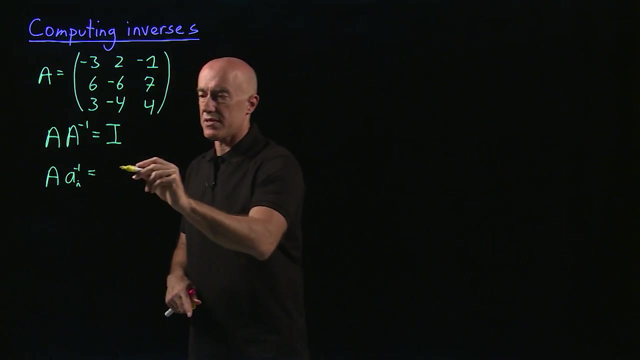 So we can view this as A multiplying, say the ith column of big A. So let me call that little a sub i inverse. So that's the ith column of big A inverse. It's equal to the ith column of the identity matrix. So this one I'll just call Ei. 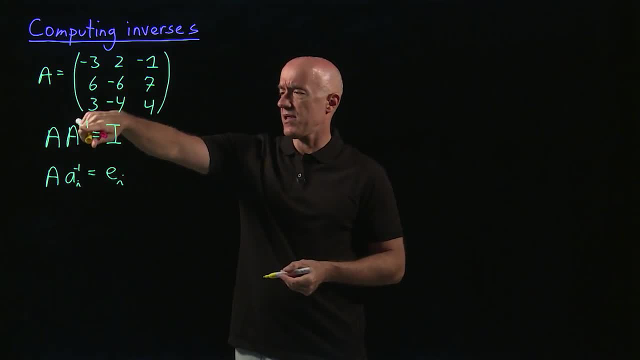 So to solve for the capital A inverse, we just need to solve n equations of this type. We can use Gaussian elimination. but it's even simpler if we just bring the matrix A to reduce row echelon form. So let me show you then what matrix then we need to work on. So we have our A matrix. 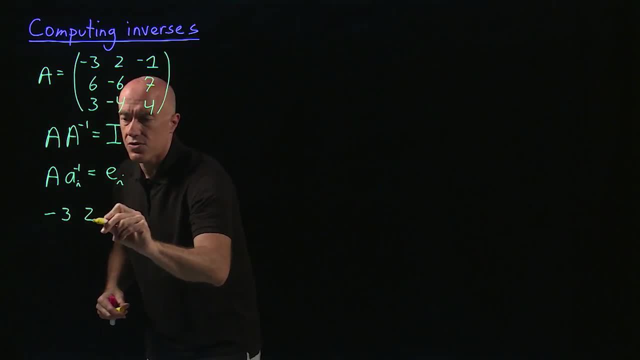 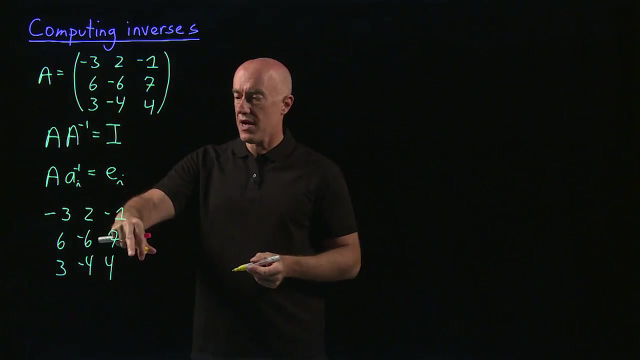 So we have minus 3, 2, minus 1, 6, minus 6, 7, 3, minus 4, 4.. And to that we attach the right hand sides, But the first column of the right hand side will be the first column. 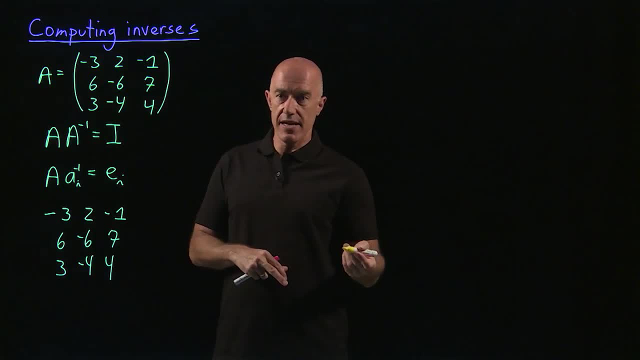 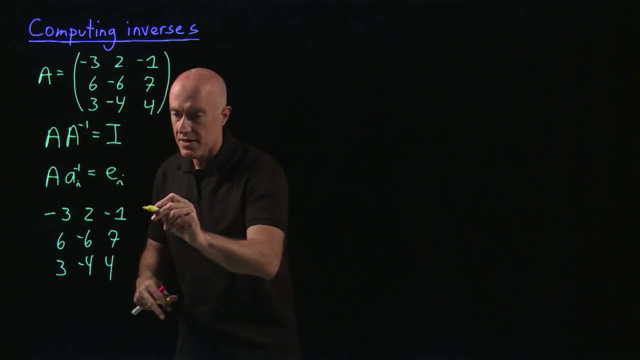 of the identity matrix, second column of the right-hand side, the second column of the identity matrix. So to the right-hand here we just attach the identity matrix. So we have 1, 0, 0, 0, 1, 0, 0,, 0, 1.. 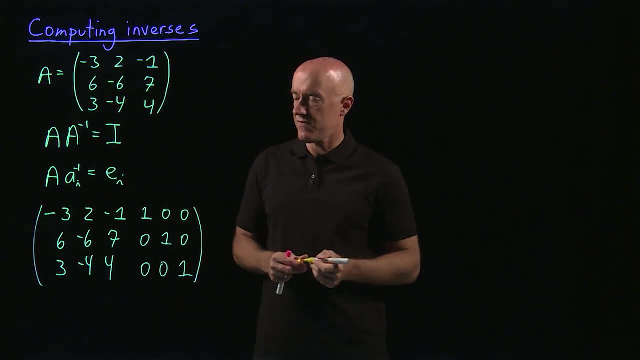 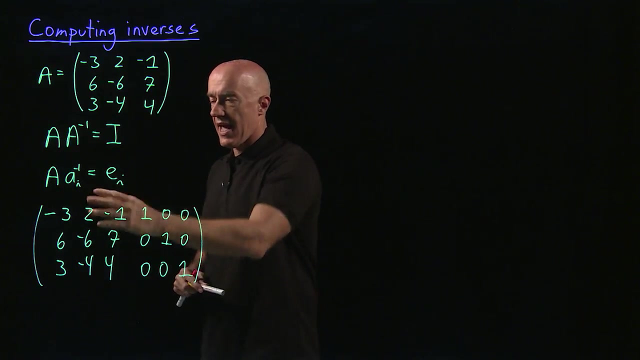 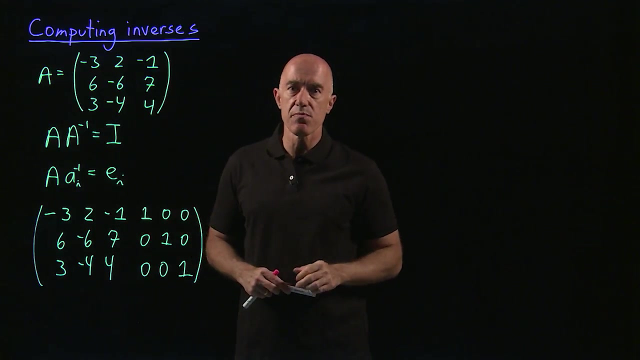 So that becomes our augmented matrix for this problem, And now the algorithm is, rather than just Gaussian elimination, we bring this A matrix here to reduce row echelon form. Then we can just read off the solution, And what that means is that as we bring the A matrix to reduce row echelon form, that will actually be the identity matrix, because this is an invertible matrix. 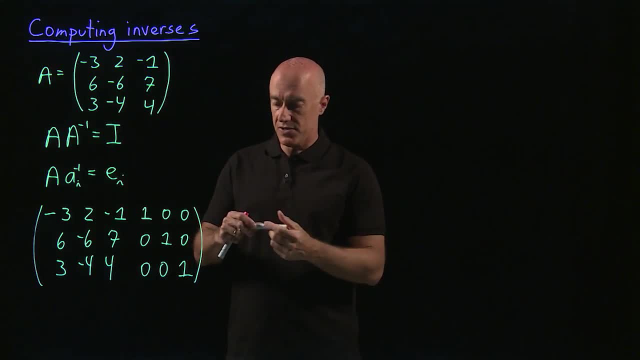 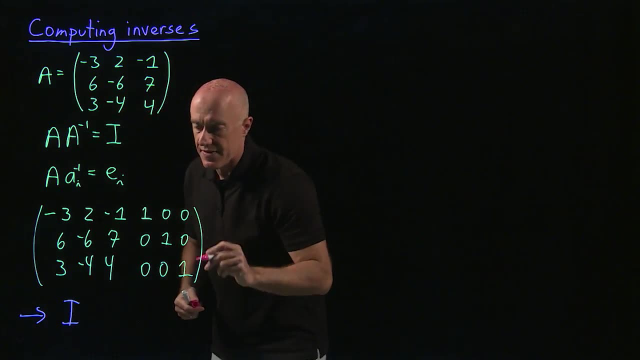 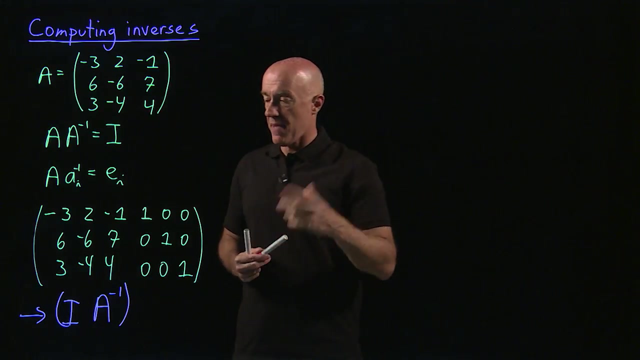 Then the right-hand side will go, So this will eventually go to the identity matrix and then the identity matrix will go to the inverse matrix. So in some sense it will be magic where we do this Gaussian elimination-like manipulation on this matrix and then out pops the inverse matrix. 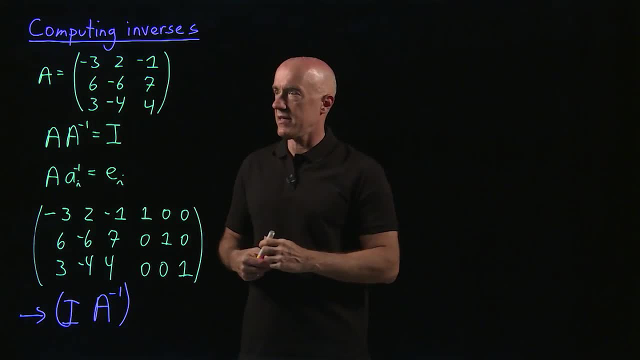 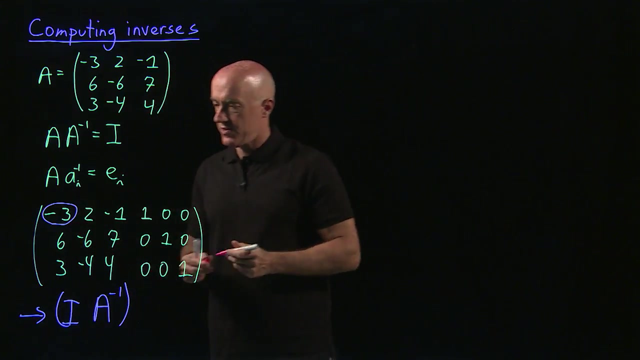 A very efficient algorithm For finding the inverse. Okay, so let's do it. To do that, we need to find our pivot. So we have our pivot. here is the minus 3. So we can eliminate everything below the pivot. 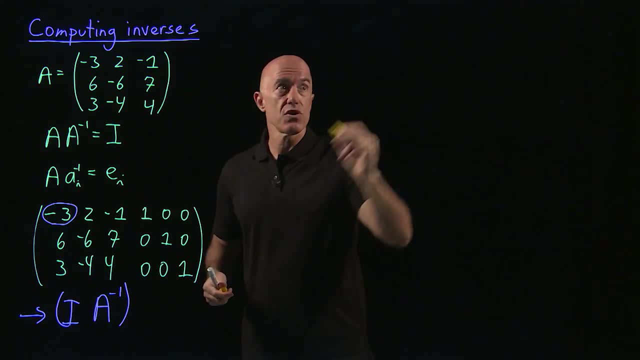 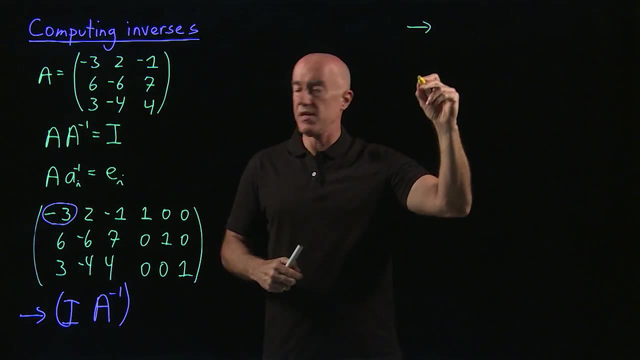 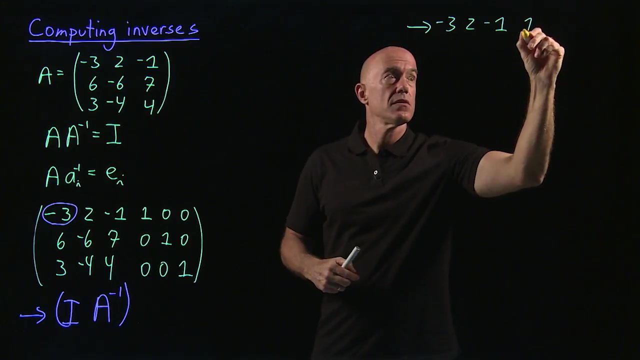 So let me this one then will go here And we have the first row minus 3, 2, 1.. 2 minus 1.. And then 1, 0, 0.. Okay, we multiply the first row. 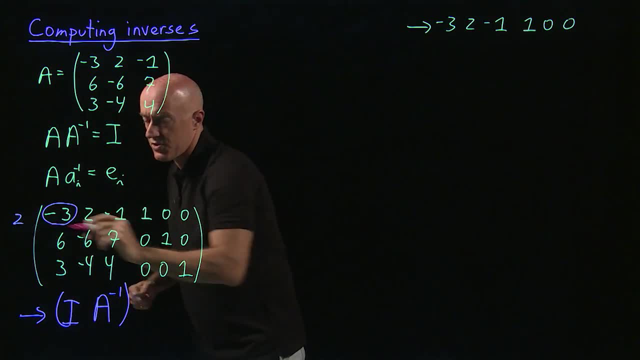 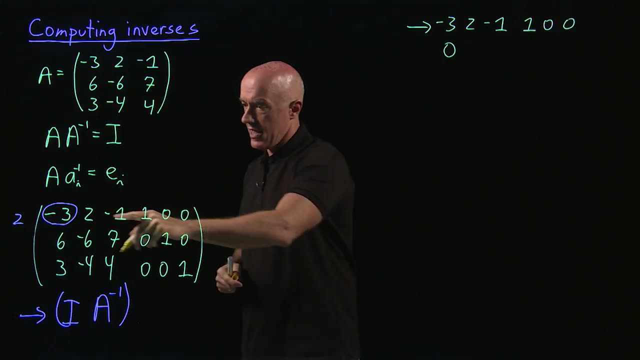 I can put the multiplier here by 2. And add it to the second row to eliminate the 6. So we have 0.. And then we have 4 minus 6 is minus 2.. We have minus 2 plus 6.. 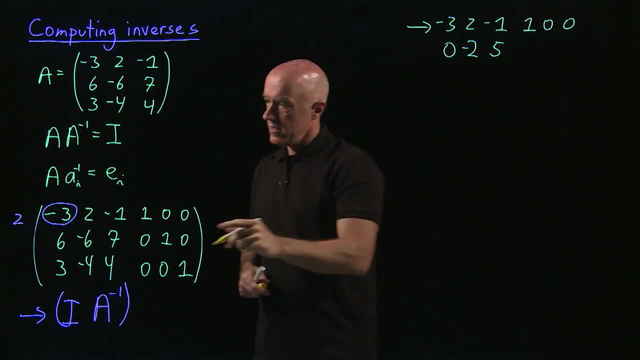 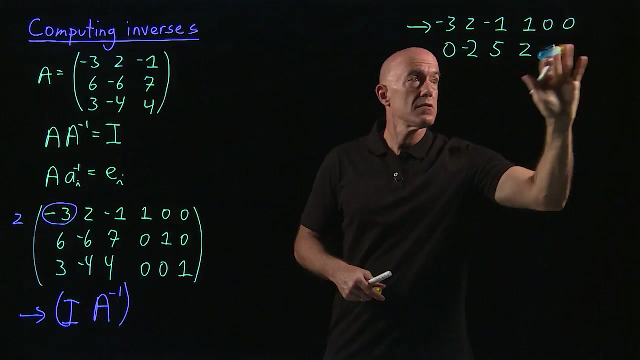 2 plus 7 is 5.. We have 2 plus 0 is 2.. We have 0 times 2 is 0. And 0 times 2 is 0. So 0, 1, 2, sorry. 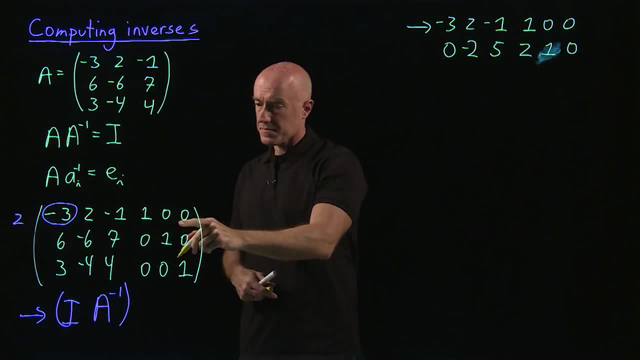 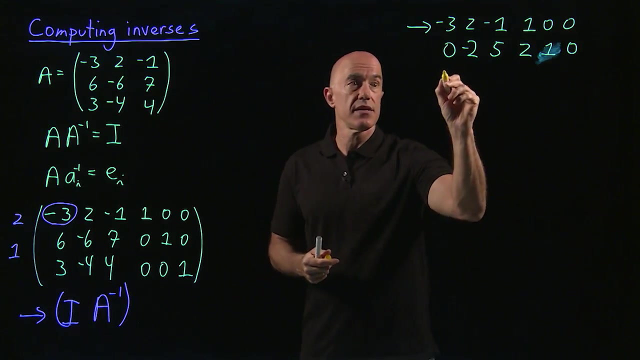 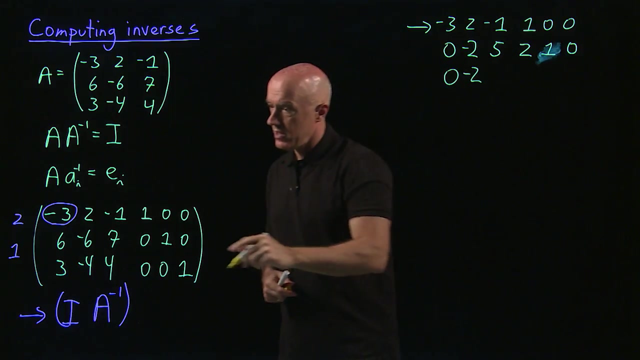 1, 0.. Okay, And then we multiply by 1 here, right? So we're just adding the first row to the last row. So then we'll get a 0 here, And then we'll have a 2 minus 4 is minus 2.. 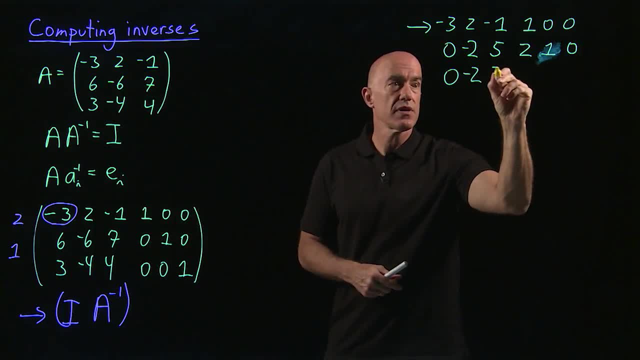 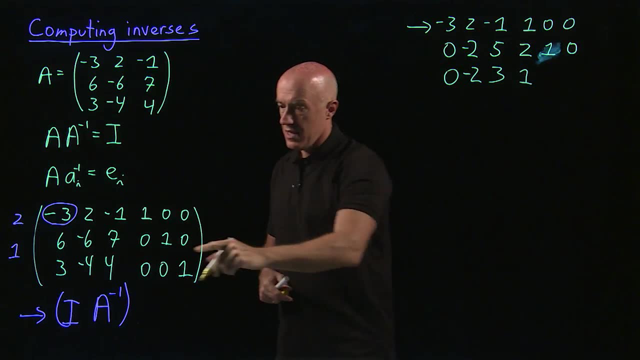 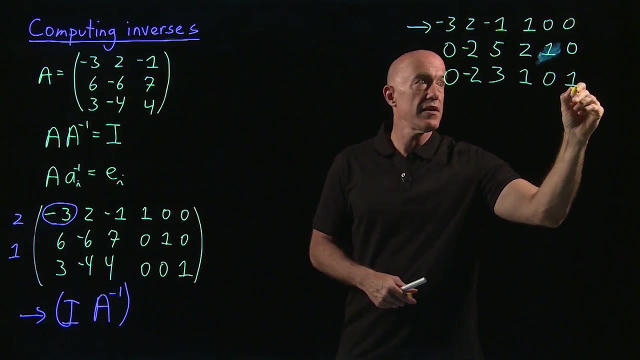 And we'll have a minus 1 plus 4 will give us a 3.. And then we'll have a 1 plus 0 will give us a 1.. A 0 plus 0 will give us a 0.. And a 0 plus 1 will give us a 1.. 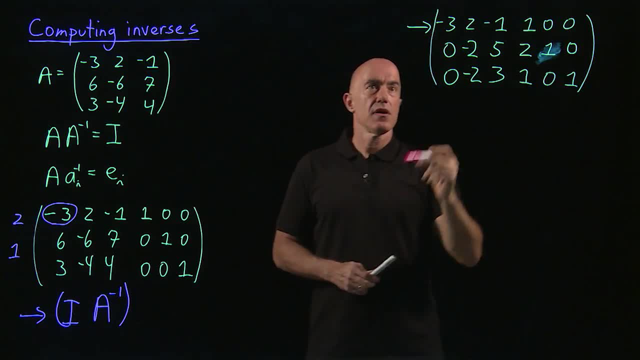 Okay, This minus 3, we're going to eventually want a 1 there, But there's no point to do that yet. Let's work on the next pivot first. So this is minus 2 is the next pivot. So we want to eliminate above and below. 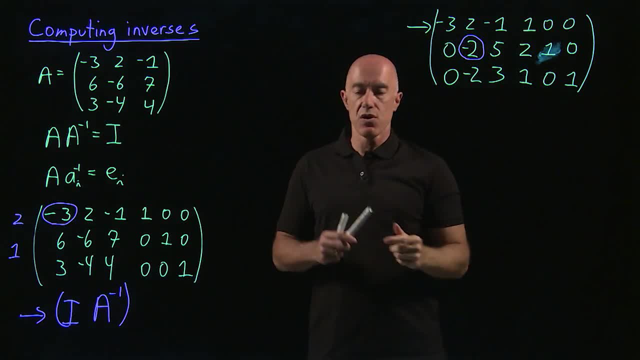 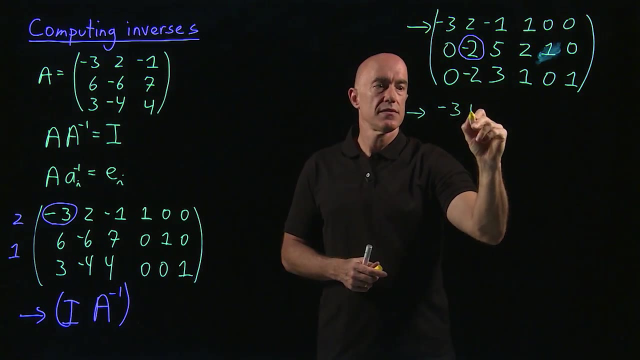 So when we go above we just add. When we go below, we subtract and we multiply by minus 1 and add, And then what do we get? So above we're just adding to the first row, So minus 3, 0.. 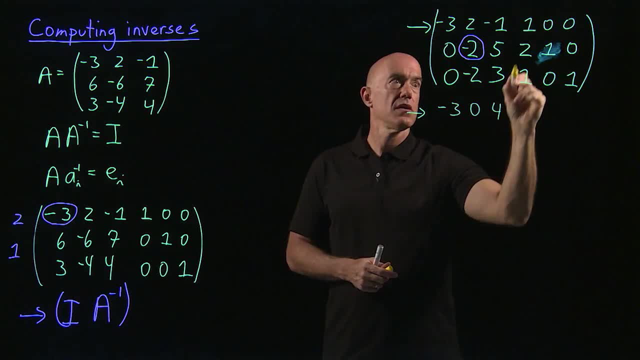 5 minus 1 is 4.. 2 plus 1 is 3.. 1 plus 0 is 1.. 0 plus 0 is 0.. The second row is just the same: 0 minus 2, 5,, 2, 1, 0.. 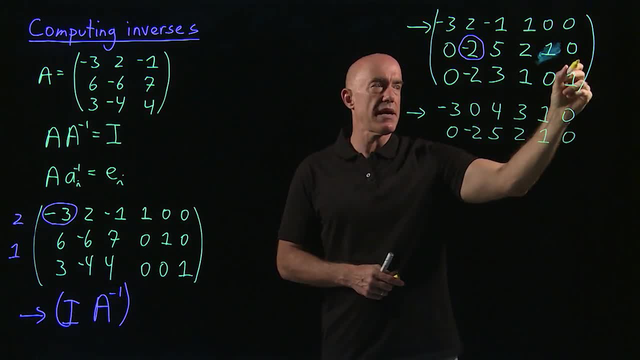 The last row. we multiply the second row by minus 1 and add it to the last row, So 0, 0.. So minus 5 plus 3 is minus 2.. Minus 2 plus 1 is minus 1.. 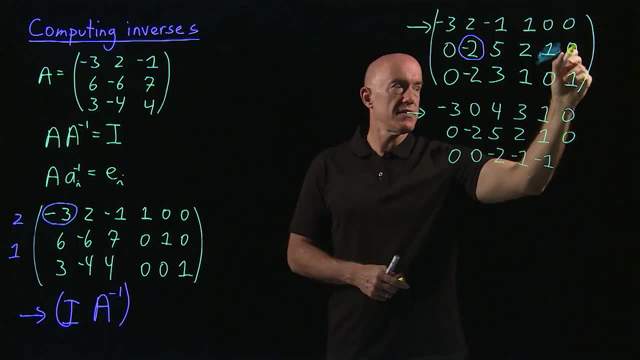 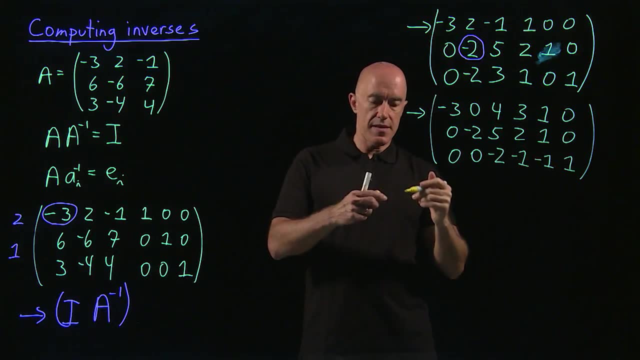 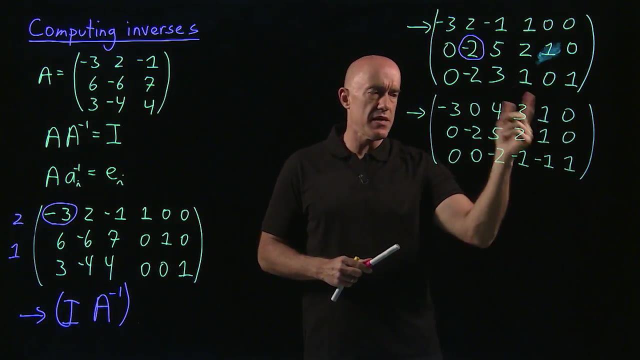 Minus 1 plus 0 is minus 1.. 0 plus 1 is 1.. OK, Now the last pivot. So sometimes it's simpler if we divide by a number. Sometimes it's harder. In this case, I won't do that. 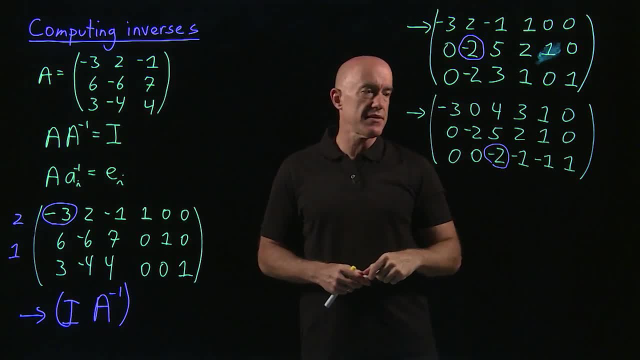 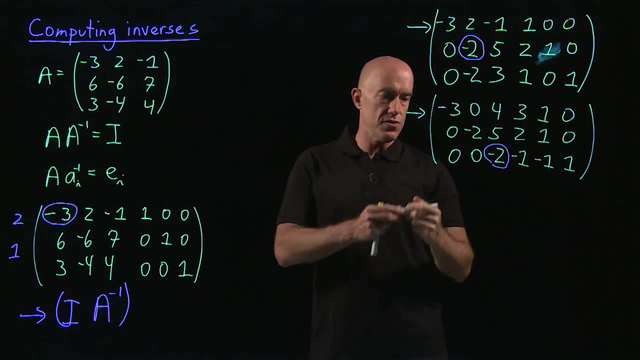 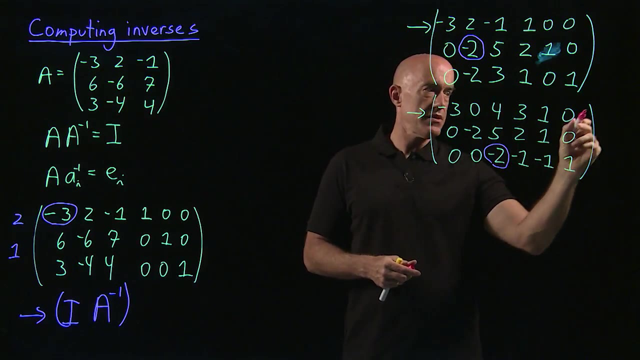 So we'll save converting these pivots to 1. We'll do in the last step, So this time I want to eliminate above the minus 2.. So the first one we're going to be multiplying by 2.. OK, 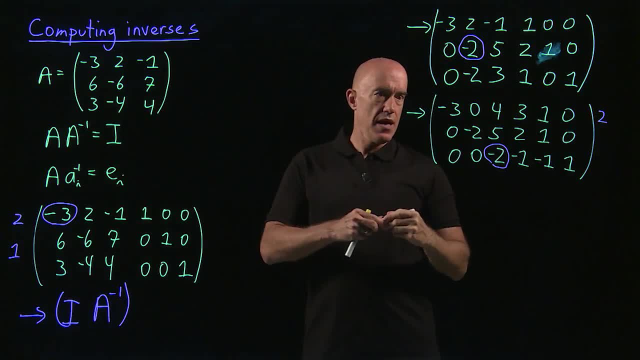 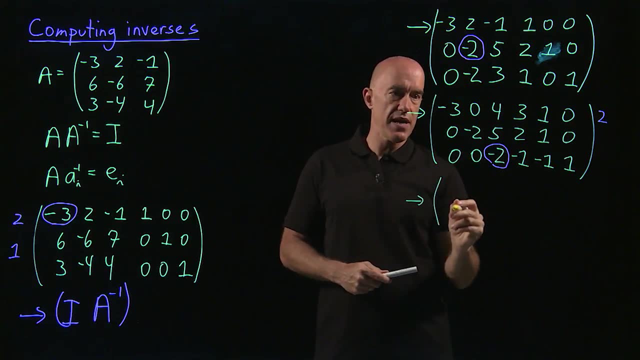 So this one multiplies by 2 for the first row. So what will this become? So the 0s here don't do anything. So we have minus 3, 0. And then we get a 0. And then we have minus 2 plus 3 is a 1.. 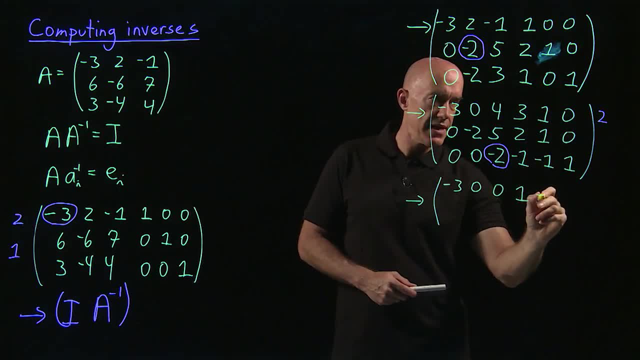 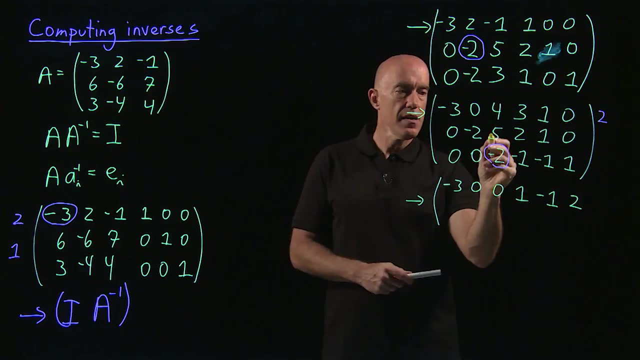 We have a minus 2 plus 1 is a minus 1.. And we have a 2 plus a 0 is a 2.. OK, Now we have to eliminate this 5.. Unfortunately, we have fractions, So it makes my life a lot harder. 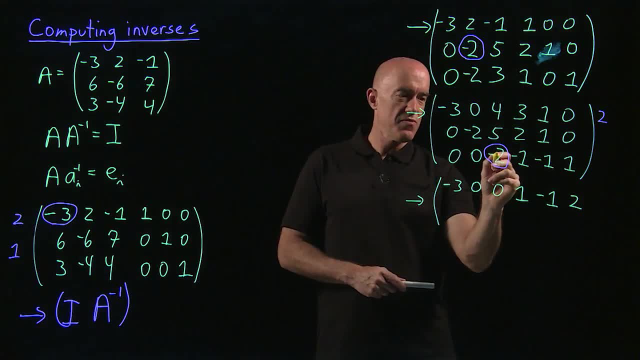 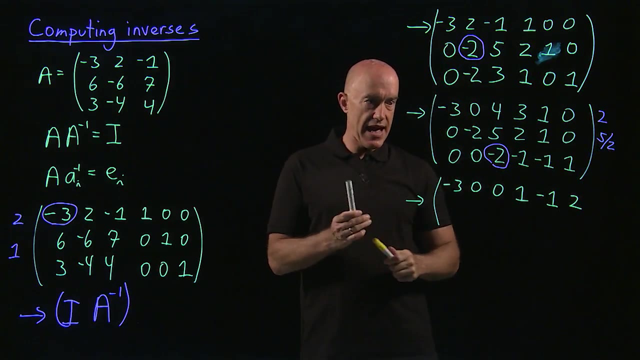 But let's see. So in order to eliminate the 5, we need to multiply by 5 divided by 2 and then add. OK, So let me write that here so we can remember. So we need to multiply the last row by 5 divided by 2 and then add. 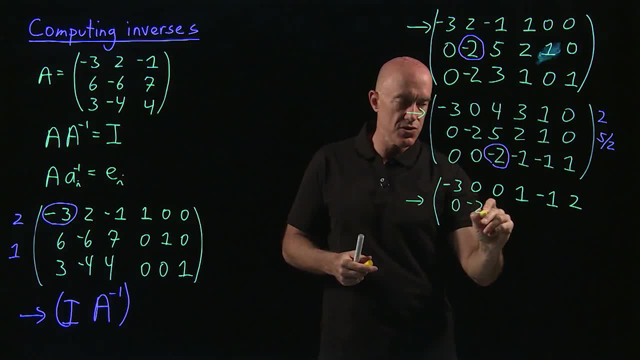 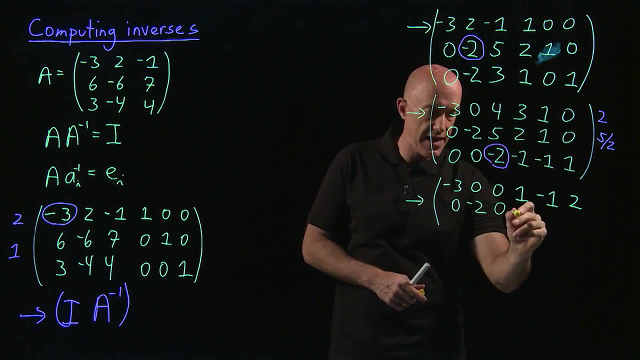 So then we'll get a 0 minus 2, 0.. So we just have a little bit of arithmetic here to do. So we got minus 5 halves plus 2.. So 2 is 4 halves Minus 5 halves. plus 4 halves is minus a half. 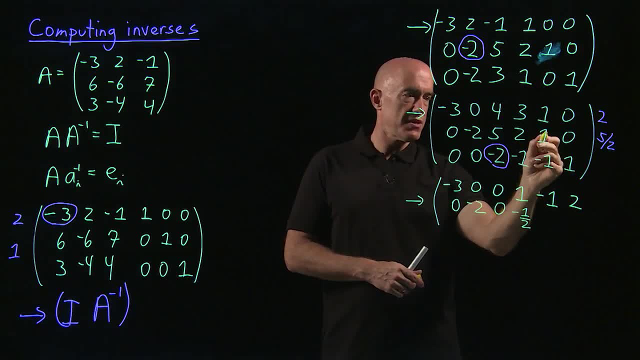 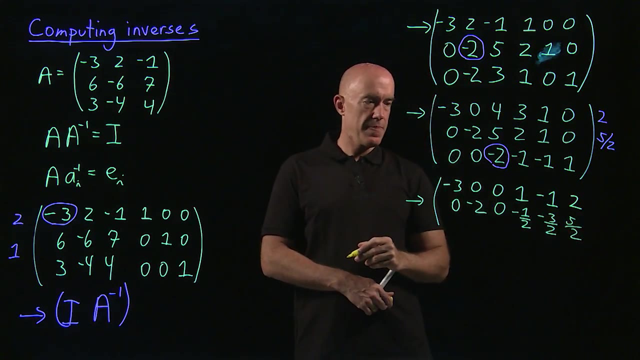 OK, Then we got minus 5 halves, plus 1 is going to be minus 3 halves, And then we've got 5 halves plus 0 will be 5 halves. OK, And then the last row is our 0 minus 2 minus 1.. 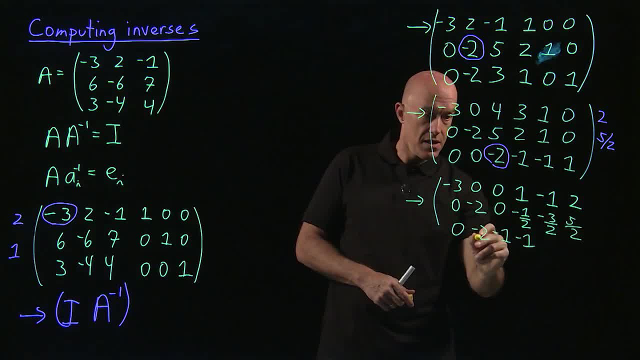 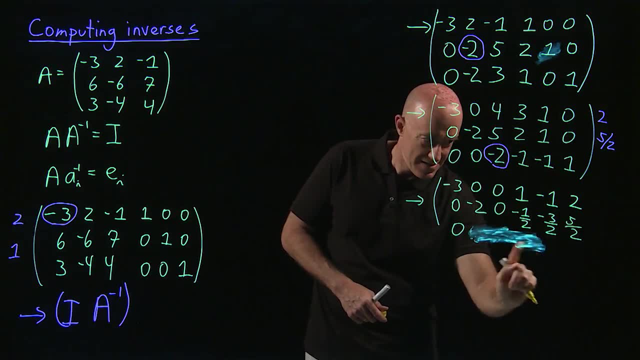 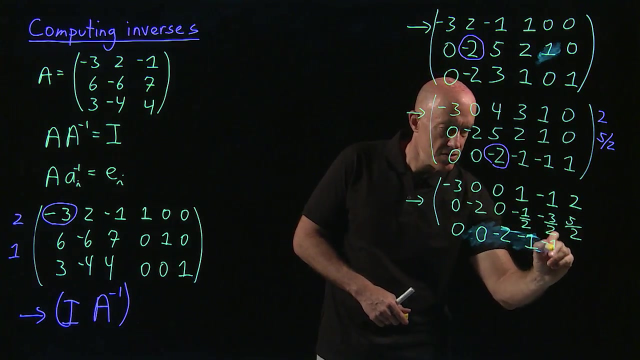 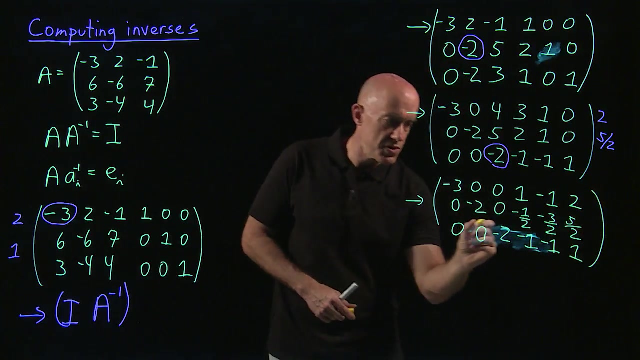 Minus 1, 0.. Whoops, Sorry, sorry, I apologize. 0, 0.. OK, And then we have a minus 2 minus 1 minus 1, 1.. OK, So I hope you can still read that over there. 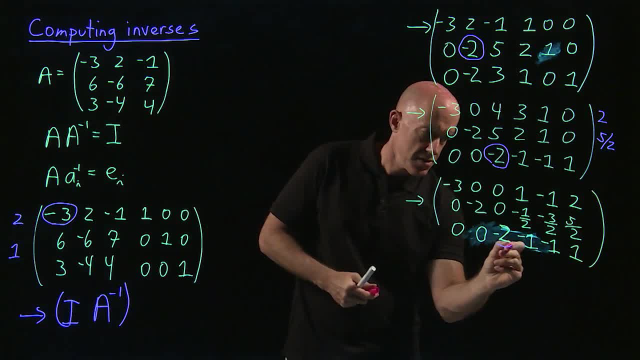 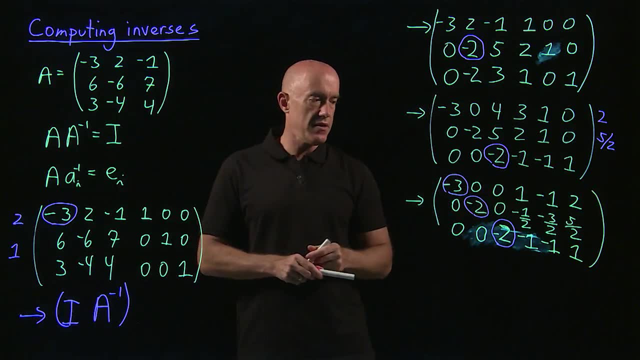 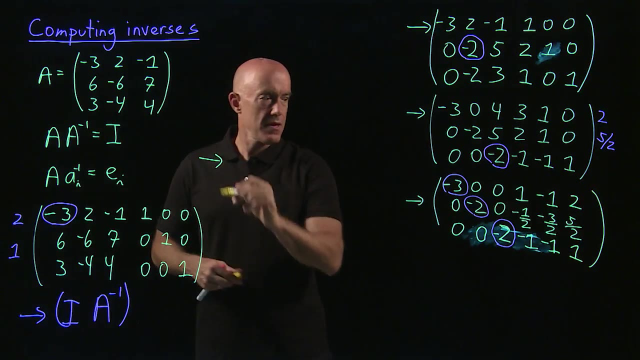 Last step: we need to this minus 2 here, this minus 2 here, this minus 3 here. we need to convert those to 1.. So let me do that here. So this is the final step. So the matrix here we divide through by minus 3.. 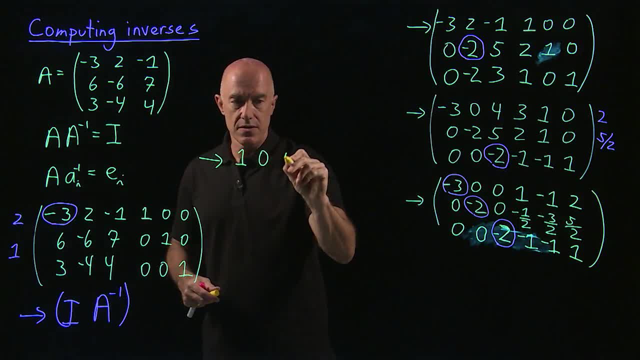 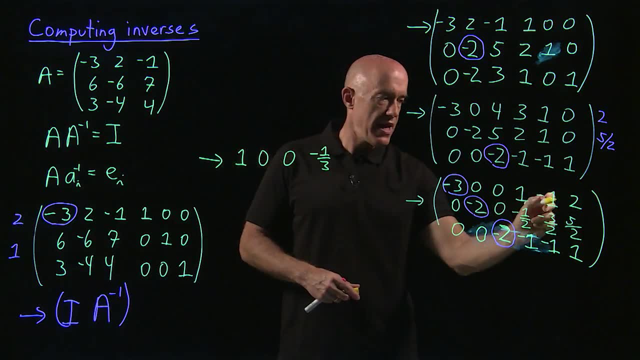 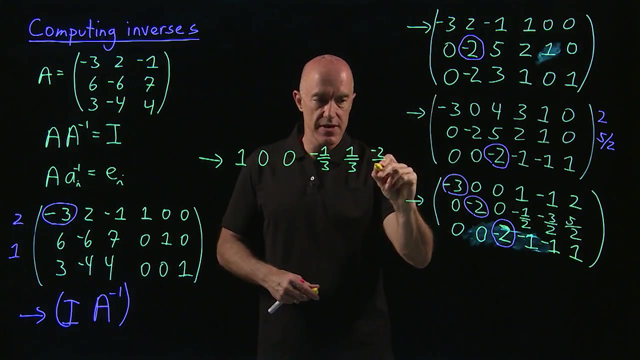 So we end up with a 1, 0, 0.. Divide through by minus 3.. So we have a minus 1 third, We have a 1 third And we have a minus 2 thirds. OK, So we have these fractions. 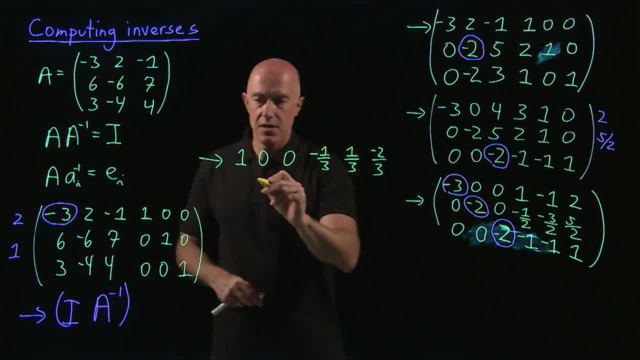 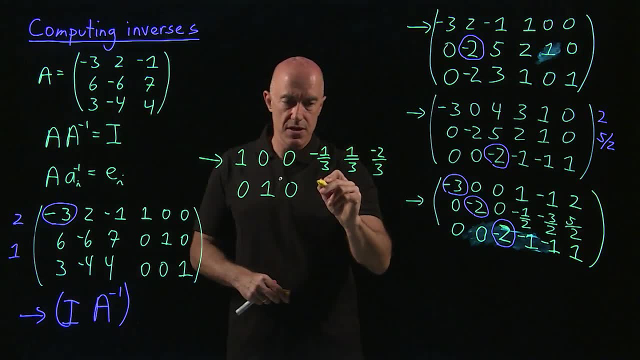 The second row. we divide through by minus 2.. So we have a 0, 1, 0,. right, We're getting the identity matrix. We divide through by minus 2.. So we have a 1 quarter. We divide through by minus 2.. 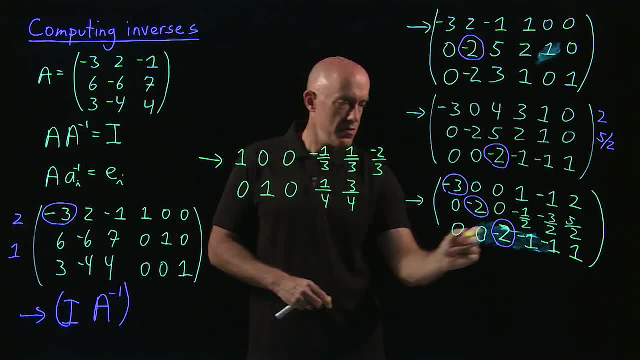 So we have a 3 quarters. We divide through by minus 2.. So we have a minus 5 quarters. OK, And then the last row: we divide through by minus 2 again, So we have 0, 0, 1.. 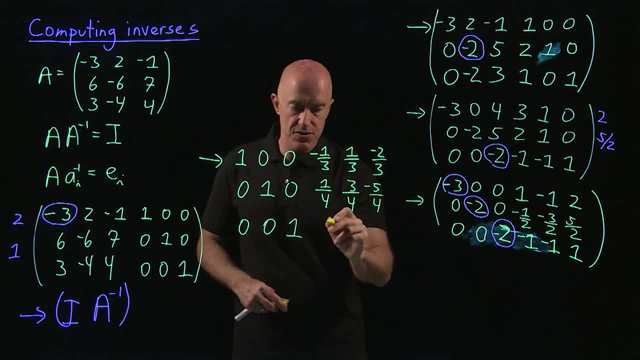 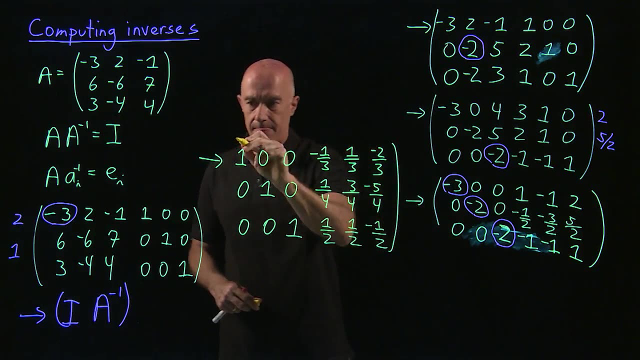 And then minus 1 divided by minus 2 is 1 half. Minus 1 divided by minus 2 is 1 half, And 1 divided by minus 2 is minus 1 half. OK, I hope I did my algebra right. 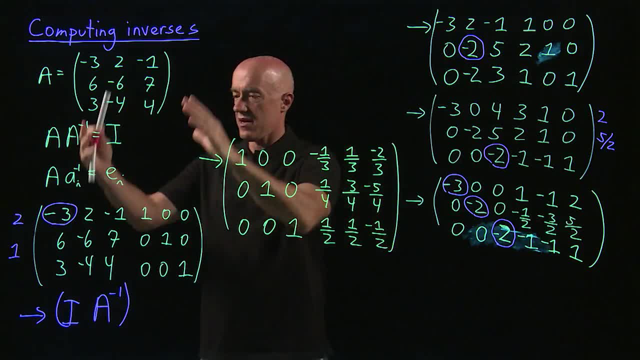 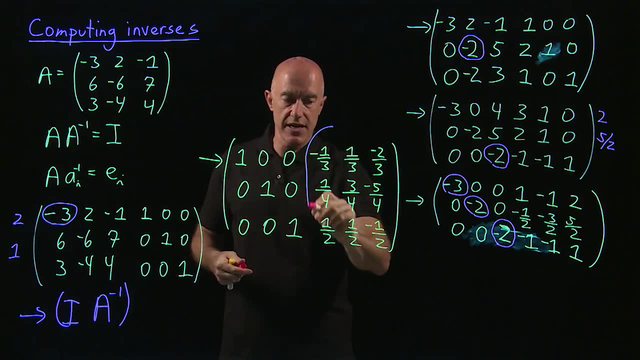 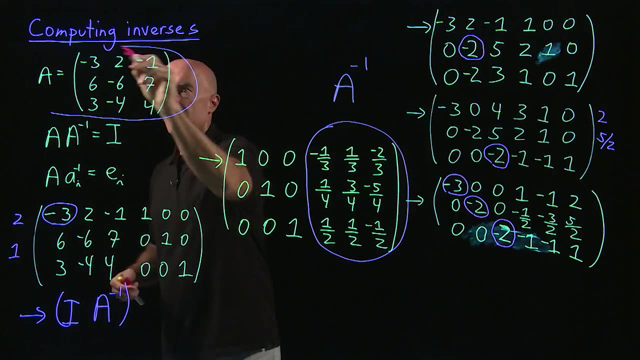 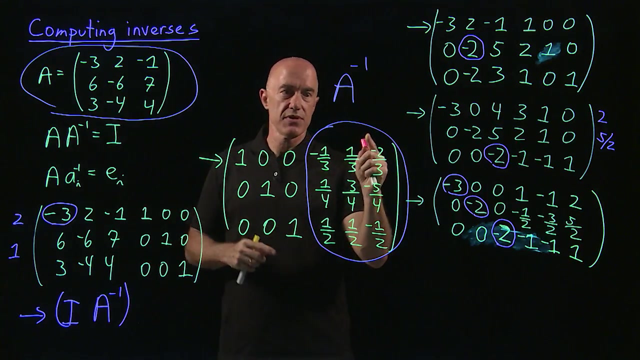 What did we do here? So we had a AI here And we converted it to IA inverse. So this matrix here Is our A inverse Right. This matrix here Was our A. So if my arithmetic was correct, Then A times A inverse will give us the identity matrix. 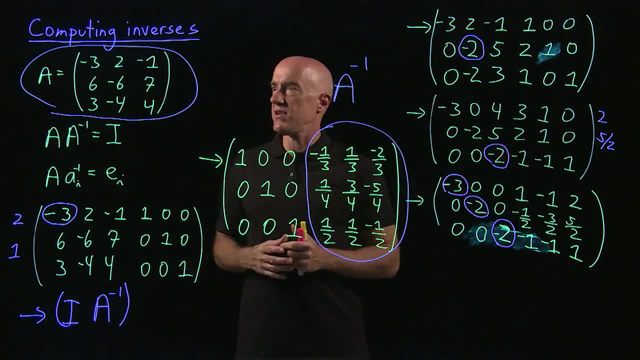 OK, So what I showed you in this video Is the algorithm of obtaining an inverse matrix When an n by n matrix is invertible. You do that by writing AI And then you bring A to reduce row echelon form And I becomes A inverse. 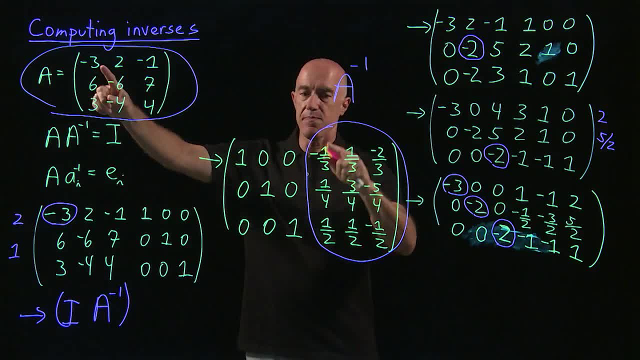 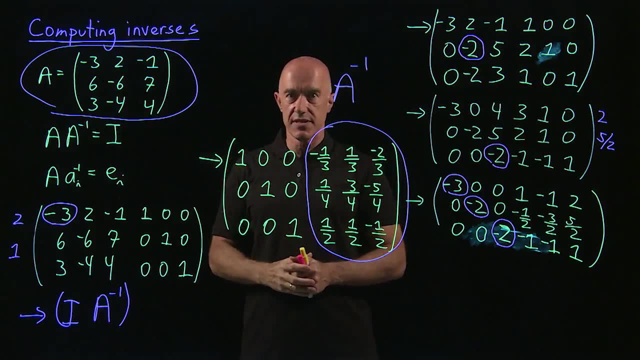 So please write this down on a piece of paper And multiply these two matrices And convince yourself That A times A inverse is equal to the identity matrix. I'm Jeff Chasnov, Thanks for watching And I'll see you in the next video. Bye. 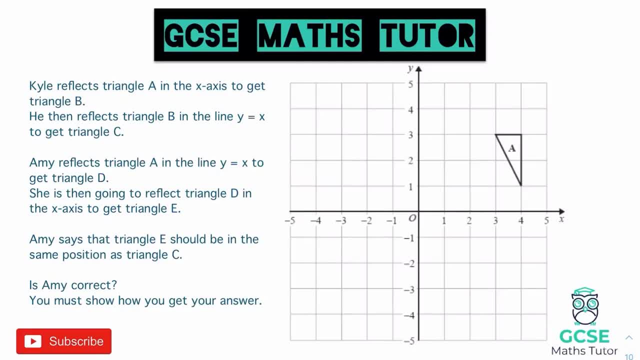 Okay, so in this video we're going to have a look at reflections. So throughout the video, we're going to have a look at reflecting shapes in different kinds of lines, whether they be horizontal, vertical or even diagonal lines, And we're also going to have a look 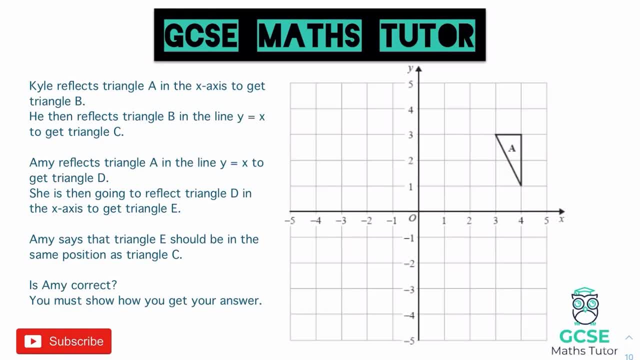 at describing those reflections as well. So we're going to be finishing up on this question that you can see on the screen, but before that we're going to obviously get into the basics and make sure that we're okay with all the elements of reflections. So with that, 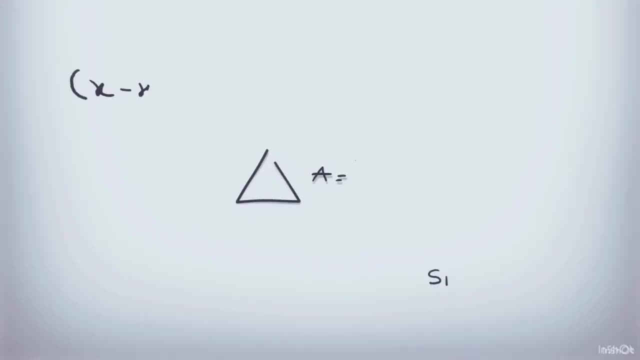 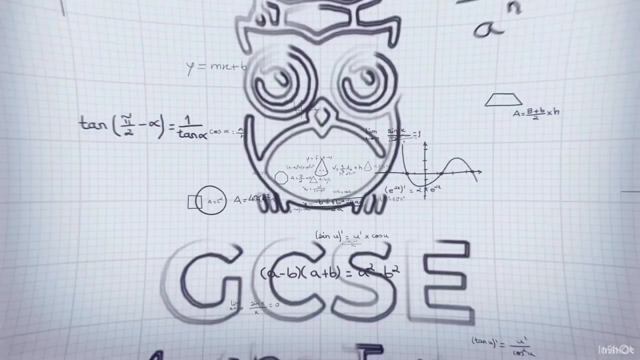 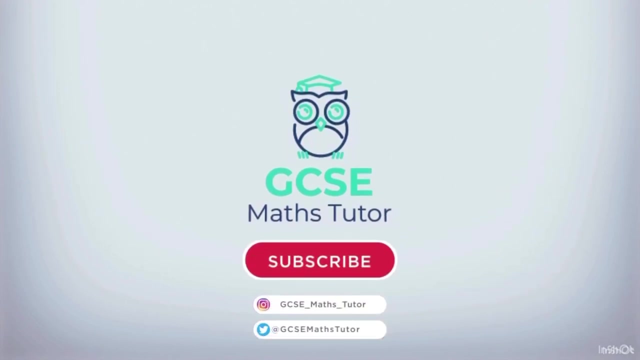 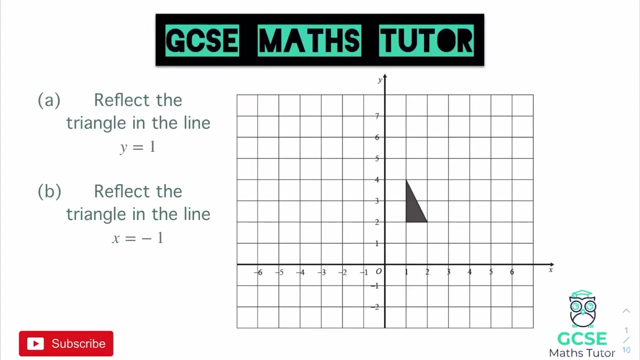 being said, let's get started. Okay, so, in order to understand a reflection, we have to understand, obviously, how to find the lines in order to reflect it. So we've got two questions here and we're going to do them both on the same grid. Now, grab a piece of paper, grab a pen, make some notes.